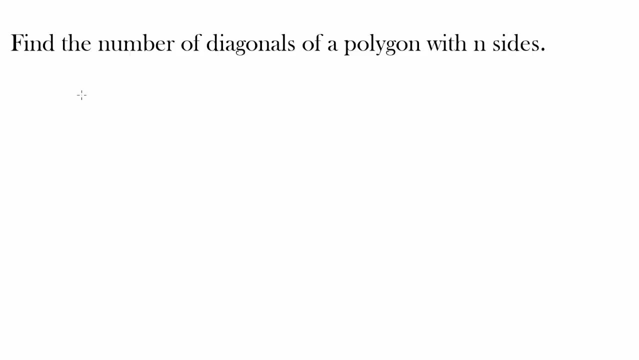 Let's say some random person comes up to you and asks you: how many, how many diagonals are there? What's the number of diagonals for the hexagon? For the hexagon, which is a polygon with six sides, So in this case, n is equal to six. n is the number of sides. So what you may do is you're going to start by drawing out a hexagon- If I can draw a hexagon- one, two, three, four, five, six- and you're going to start drawing diagonals. That's. 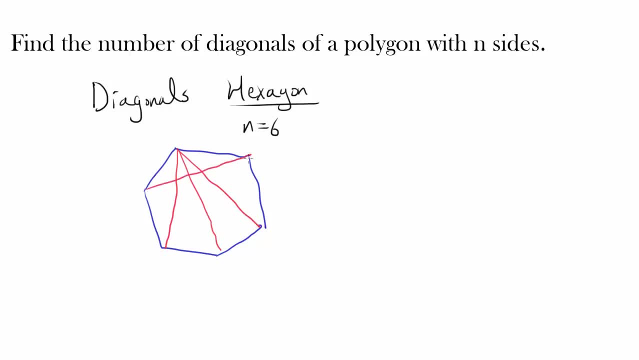 one, that's two, that's three, that's four, that's five, that's six, that's seven and you're going to try hard not to mess up- That's eight- we are missing this one- and that's nine. So you're going to say: hey, there's nine diagonals for the hexagon. Let's say another person comes up to you and he or she says: hexagon is too boring, How about the polygon with 100 sides? So he's going to give you some polygon with 100 sides. I'm not going to take that. 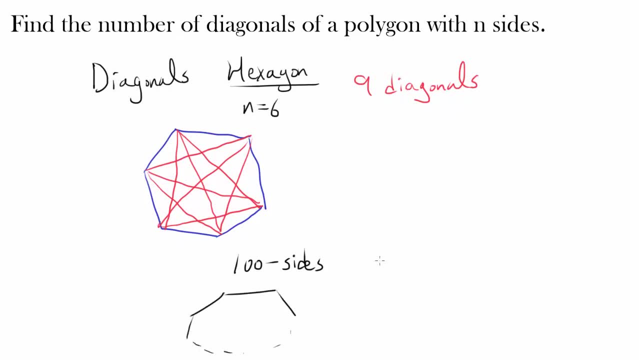 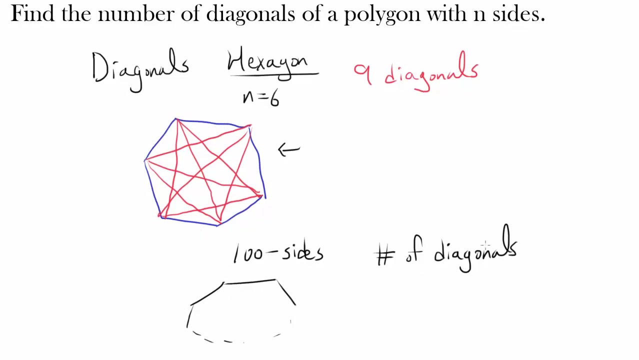 It's going to have a lot of sides And he's going to ask you: what is the number of diagonals? now, What is the number of diagonals in this case? And you're going to fumble if you try to do it the same way, because that's going to take you a long time for you to draw out the polygon precisely And it's going to take a long time once again to count each diagonal. So how can you count this quickly and systematically? Hmm, that's an interesting question. 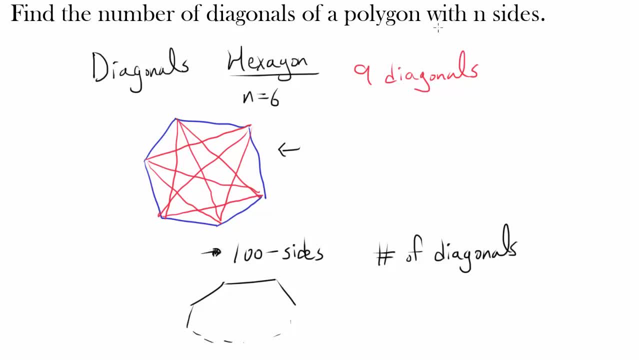 So, before we look at 100 sides or even any n sides, let's first focus on the case for the hexagon. So how can we count this nine in a quicker and better way? So let me start by drawing a hexagon. Well, let's look at, let's simplify it. Let's look at it from vortex to vortex. From this vortex, you can draw three diagonals: one to this one, one to this one and one to this one. How about from this vortex? How many diagonals? 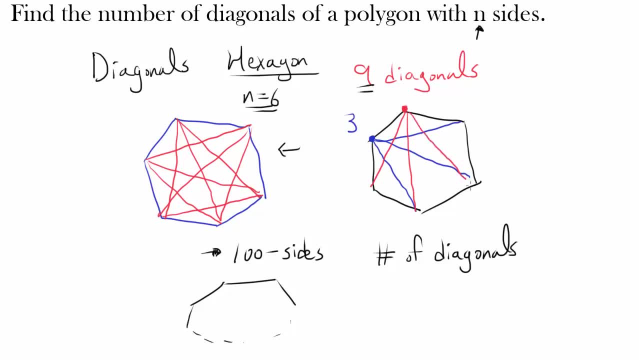 Can you draw? Well, you can draw three of them: one to this one, one to this one, one to this one. How about for this vortex? Well, you can draw three of them. once again, 123. And you're going to be able to draw three to every single one, because there's nothing special about any vertices, you're just drawing diagonals to the opposite point. So, for each, for each vortex, you're going to be able to draw three diagonals. So you may say: Oh, you can draw three times six. 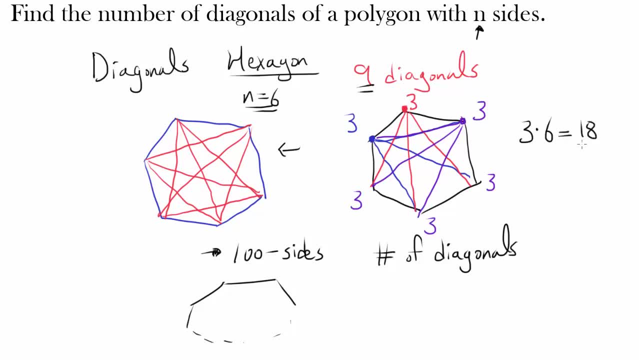 diagonals, which is 18.. But the answer is not 18.. The answer is nine. And you may say: why are we getting nine? Well, let's focus on, let's focus on this diagonal, Let's focus on this diagonal. You're counting it once, going from this vortex. you're counting it once, going from this vortex, but you're counting it one more time, going the opposite way, going from this vortex. So each diagonal is getting counted twice, one from one starting point and the other from the opposite point. 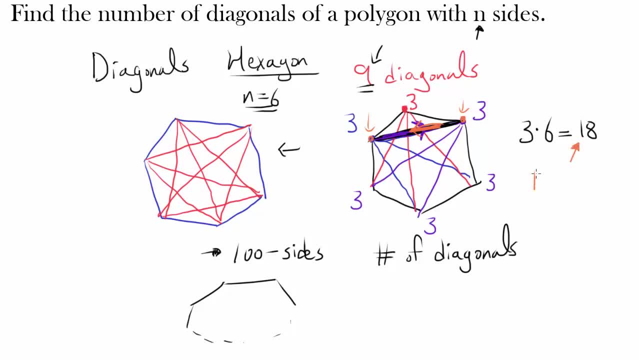 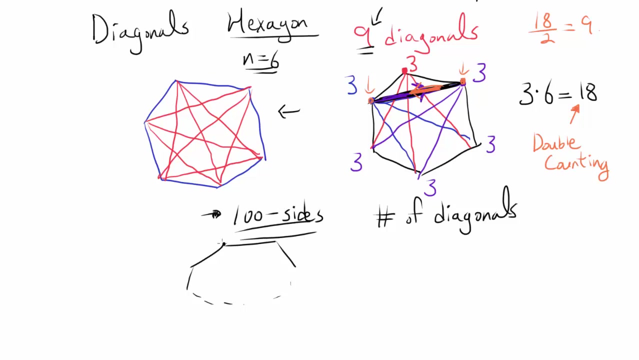 So you are double counting the diagonals when you're saying 18.. That's double counting. So to get the actual number of diagonals, you want to divide by two. So 18 divided by two is going to get us nine. Okay, so that's a quicker way of finding number of diagonals without drawing everything out. So let's try to do the same with the polygon with 100 sides. So how many diagonals can you draw? starting this point, Huh. 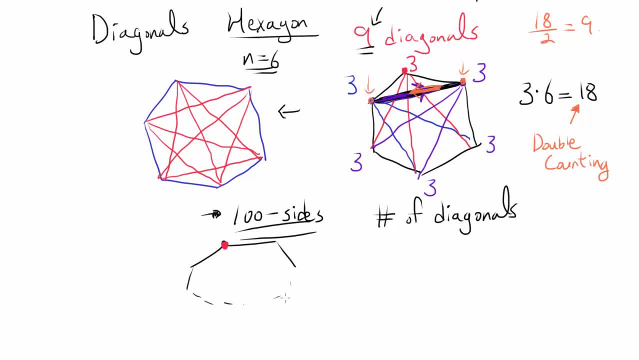 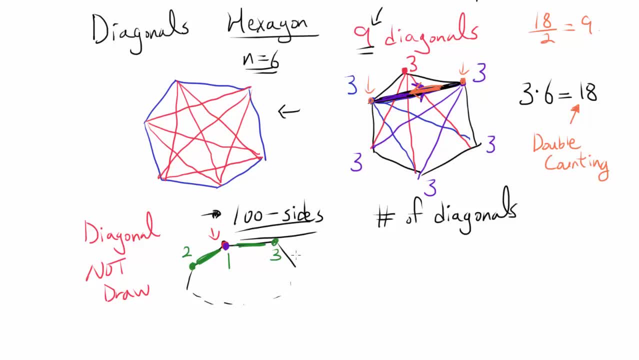 there are three diagonals you cannot draw, but there's 100 points and you cannot go to three of them. so you must be able to draw diagonals to 97 of them, 100 minus 3. so you can draw a diagonal to this one, this one and this one, and there's 97 vertices you can draw diagonal to. let me recap: 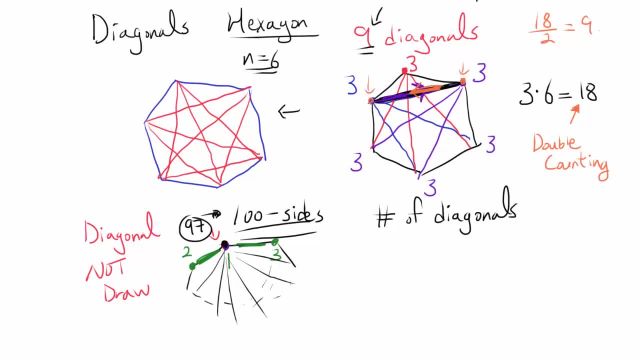 because that's very important. you have 100 points. you can get to starting this point and you don't want to go to the same point, all the points next to it, so you want to take away 3 from 100 to get 97 and that's going to apply for every single point. you can draw 97 from this point, 97 from: 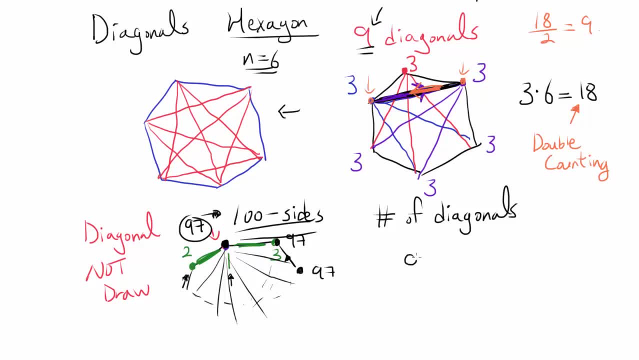 this point, 97 from this point, and so on. so you're going to have 97 times 100 diagonals. but once again, you're double counting. for every single, for every single diagonal. you're counting it once. you're counting it once from this point and you're counting it once from this point. 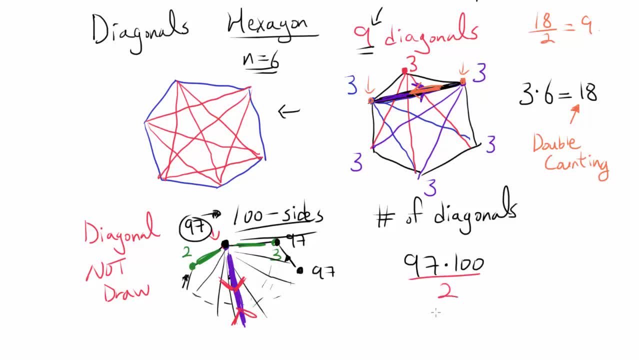 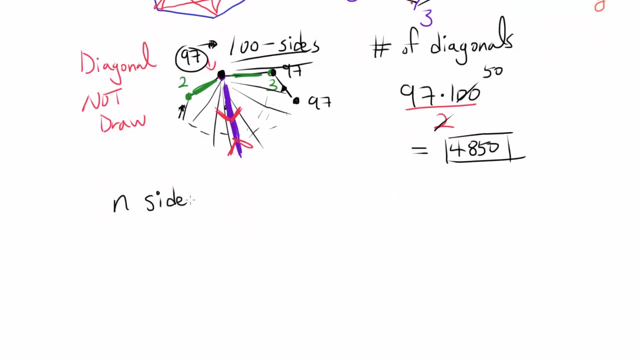 so you have to divide by 2 to prevent double counting, and this is actually going to get you 48, 50 as the number of diagonals. so how about now? let's extend it one more time. how about the polygon with n size? just some random integer, n greater or equal to 3? how many diagonals can you draw? well, let's try to. 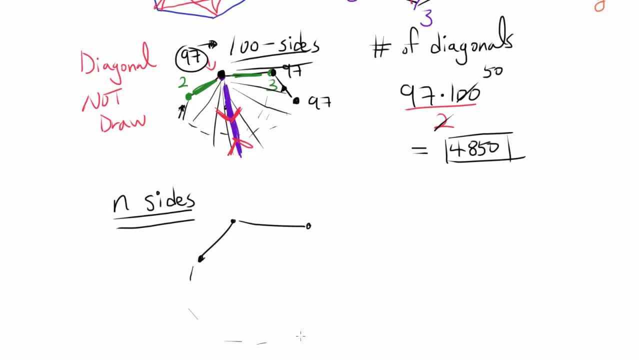 apply the same reasoning: you're going to have n size, so you're going to have n size and 48, 50 as the number of diagonals. so how about now let's extend it one more time. how about the Simon Ge degrading n age as a value? so, for example, if this条 an 0.0 value y and since 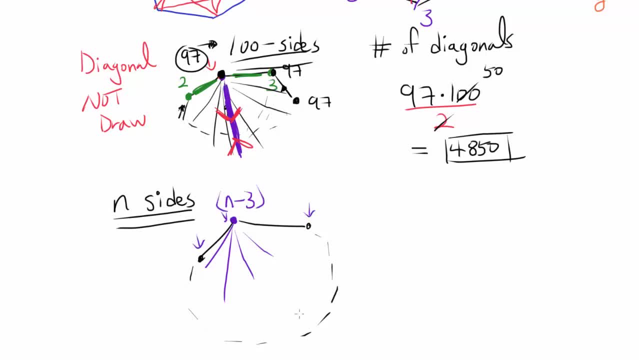 it's equal to 10, 34.. shout out a day. So from each Vertex, you can draw diagonals to n minus 3 of them. and minus 3 of them. because you cannot, merchants, because you cannot draw it to this point, you cannot throw it to this Point, over this point. and since you have an�m of them, you must be able to draw, you must be able to draw it to n minus 3 of them. so that's going to be an minus 3 for this one and minus 3 for this one. and m Newton, we're telling you something, and once. six, particlaryивdadn and Sjaoyang. again you're bitter. we're counting it, I ignore. so you want to divide, dividing by only рав göz, par Walden's Prose and find outатели. And once again you're doubling it's diagonal. so you want to divide A word right.